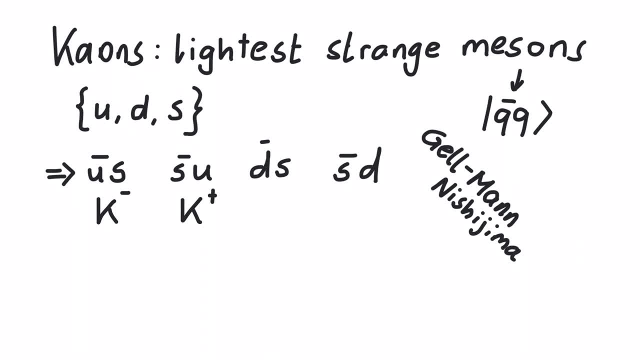 we can assign these quark-antiquark combinations to particles. These are called strong eigenstates, since they are created via strong interactions. Kaons are pseudo-scalar particles, that is, they pick up a negative sign when we apply the parity operator. As for charge conjugation, particles change. 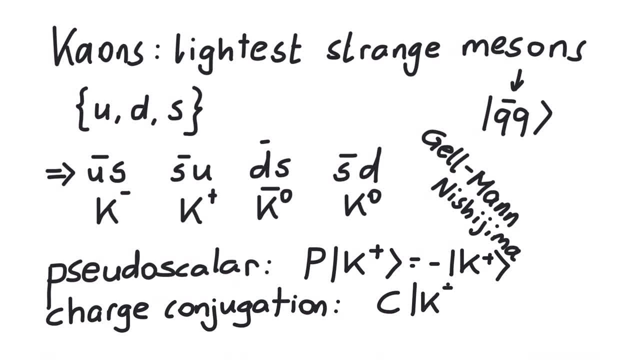 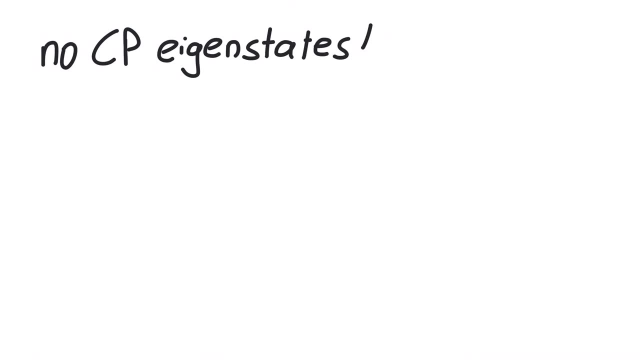 their antiparticles. so k plus goes to k minus, k zero goes to k bar zero and vice versa. The sign here can be chosen arbitrarily and has no impact on the following physics. It is important to notice that the kaons so far as described by their quark structure. 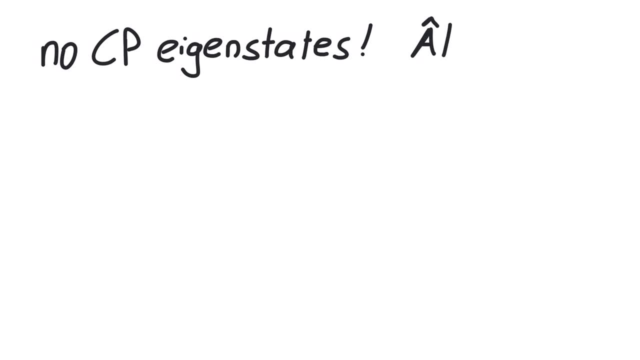 are no CP eigenstates. For an eigenvalue equation, a state has to appear on both sides of the equation. In the following we will only focus on the electrically neutral kaons and construct such CP eigenstates. Let's define a new state, k one, as the difference between k zero and 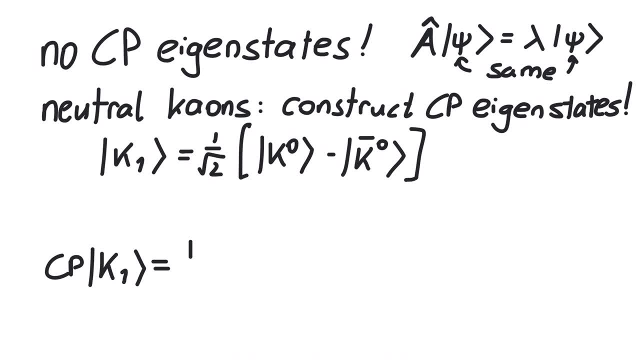 k bar zero. A CP transformation exchanges k zero with its antiparticle, while picking up a minus sign. This gives us k one again, hence this is an eigenstate. A similar calculation for k two shows that it is as well an eigenstate, but with negative. 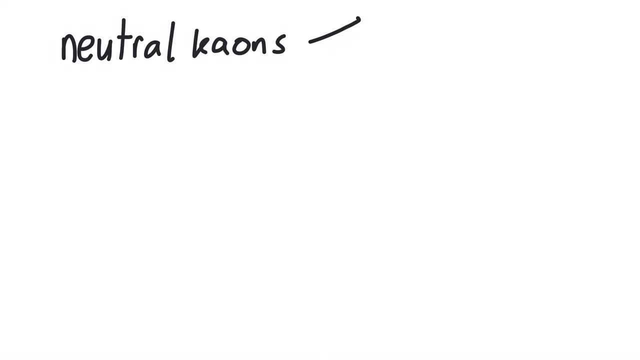 eigenvalue. Neutral kaons mainly decay via weak interactions into two or three pions. Pions are the lightest mesons. They consist only of up and down quarks. Each pion has a CP eigenvalue of minus one. If we assume weak interactions to be invariant under CP transformations. 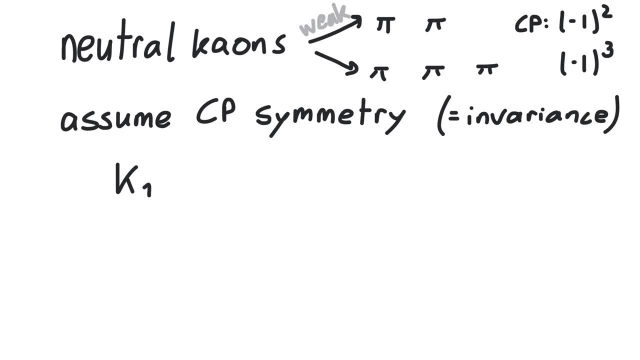 then the CP eigenvalue doesn't get changed during a weak decay. Therefore, the k one can only decay into two pions and the k two only into three. This way we have the same CP eigenvalue. This means that the k one can also decay into two pions. We just change the. 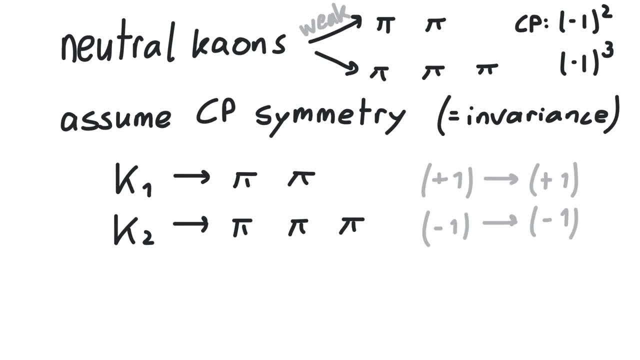 eigenvalue on both sides of the equation. K1 and K2 are called CP eigenstates. But what about experimental findings? As it turns out, three pions have approximately the same mass as one kaon, so there's only a small range for the 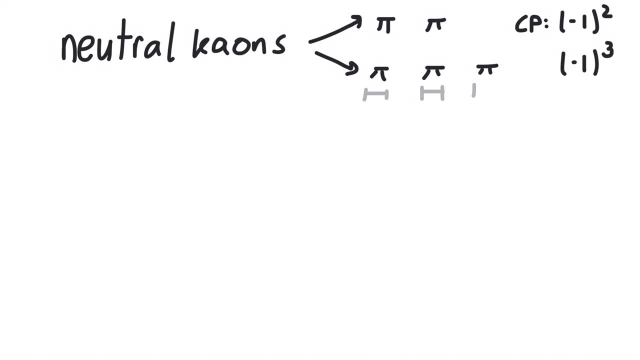 kinetic energy of the resulting pions, which prevents this process to happen. often, For a decay into two pions, their kinetic energy can be in a much wider range, rendering this process more probable. For this reason, experimentalists see two types of kaons in the lab: a short-lived one called K-short, and a. 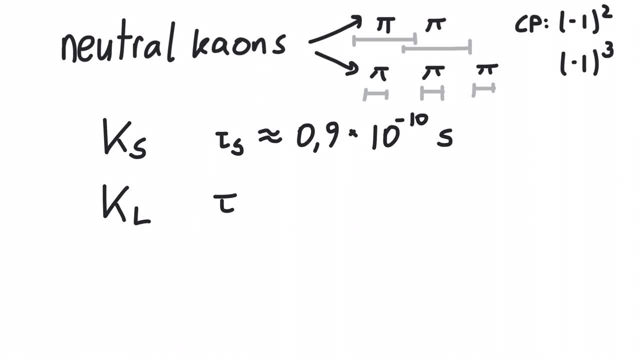 long-lived one called K-long, which lives approximately 600 times longer than its partner. The propagation in the lab tells us that they have a well-defined mass, since time evolution in quantum mechanics is, in the simplest case, due to an imaginary phase, depending on the energy which relates to the mass. Let's 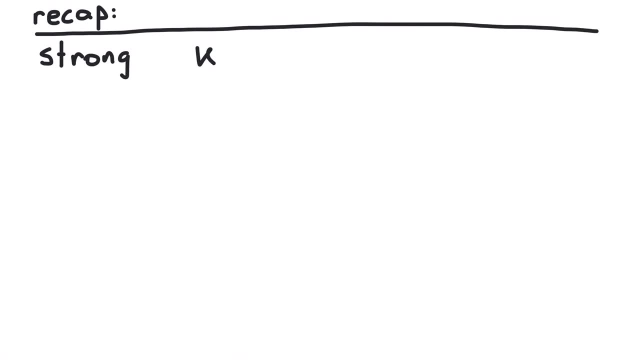 recap, We're looking at neutral kaons in three different basis systems. We have the strong eigenstates, based on their quark structure. Next, the CP eigenstates, which we constructed to fulfill CP eigenvalue equations. Finally, the mass eigenstates, having a well-defined mass in order to be the ones that propagate. 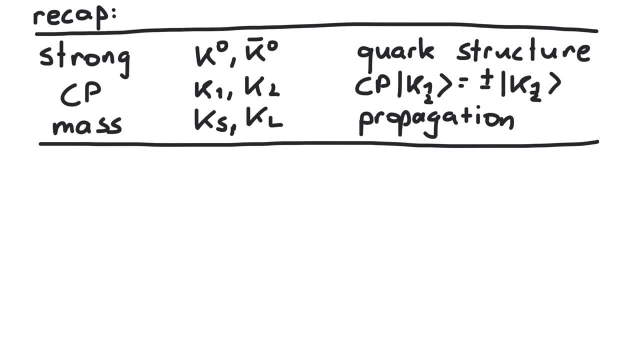 How are the mass eigenstates related to the others? Remember that K1 and K2 are distinguished by the number of pions they decay into. We also know that a decay into three pions is not very likely to happen, so it makes sense to identify K1 with K-short and K2 with K-long. This means that K-short and 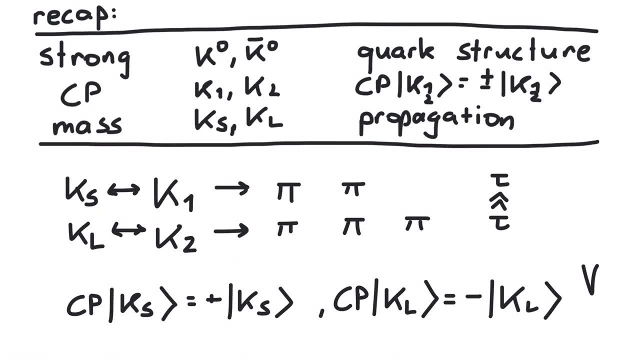 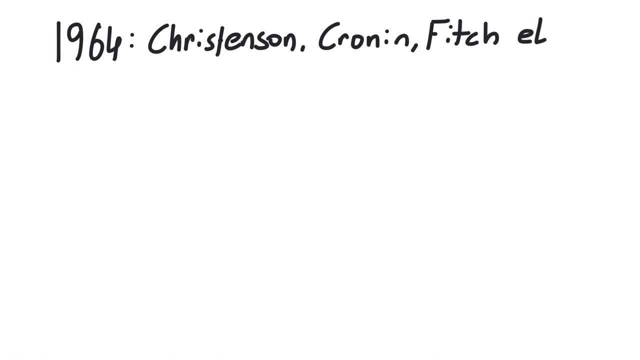 K-long must be CP eigenstates with the same eigenvalues as K1 and K2.. In 1964, Christensen, Cronin, Fitch and others performed the following experiment: They let a neutral kaon beam propagate in a long tube. Since the K-long travels. 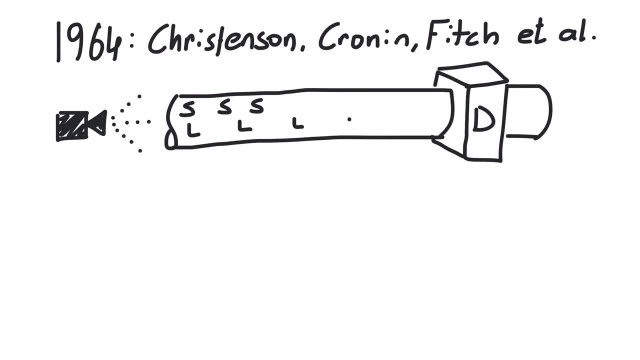 much farther than the K-short. they arrived at an arbitrarily pure K-long beam. when reaching the detector, Much to their surprise, they sometimes measured a decay into two pions. This means that a K-long decayed into two pions and the CP. 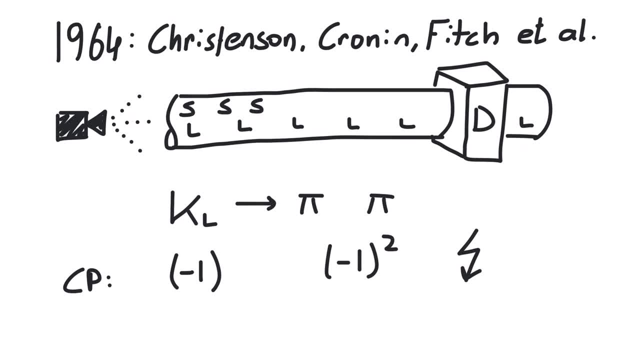 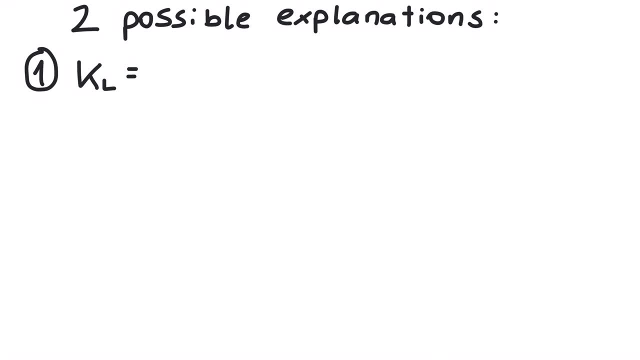 eigenvalue on both sides of the equation didn't match up. Nowadays, we have two possible explanations for this. First, we could just accept the fact that a K-long- that is a K2, can decay weakly not only into three but also into two pions. This would violate CP symmetry in. 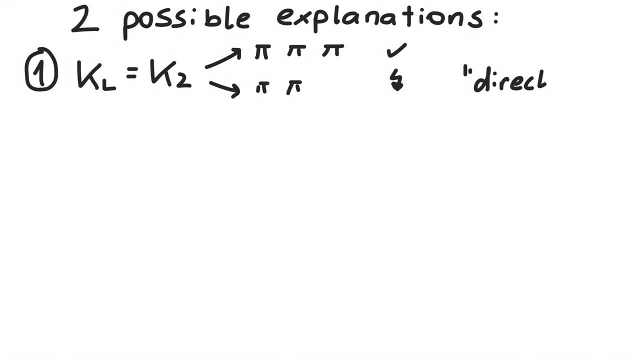 weak interactions and we call this the direct CP violation, because K2 clearly has a CP eigenvalue of minus one and two pions certainly have a CP eigenvalue of plus one. Or secondly, we redefine the propagating states K-long and K-short, to 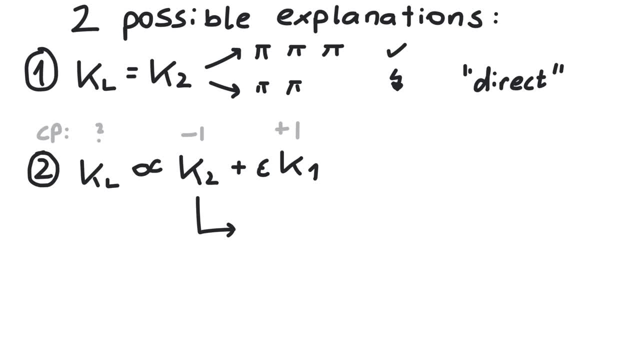 include a small part of the other CP eigenstate, Then the K-long can mostly decay into three pions, and the CP eigenvalue of the other Cp eigenstate can decay into two pions, but also sometimes into two. However, this way, k long is no longer a CP eigenstate.